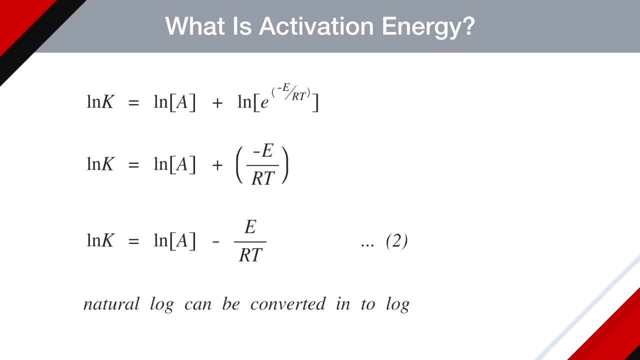 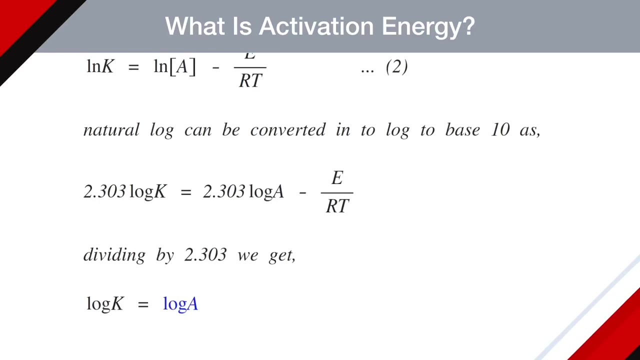 Here natural logs can be converted into log to base 10, as 2.303 log of k is equals to 2.303 log of a minus e by RT. Thus, dividing by 2.303, we get: log of k is equals to log of a minus e. 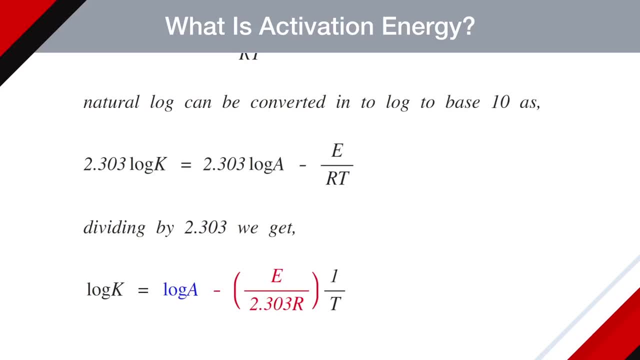 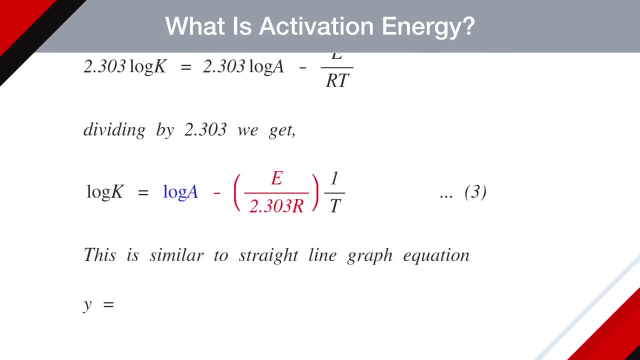 by 2.303 r into 1 by T. This is equation number three. This is similar to Straight Line Graph equation which is y is equals to mx plus c or C plus mx. So if you plot a graph of log of k, 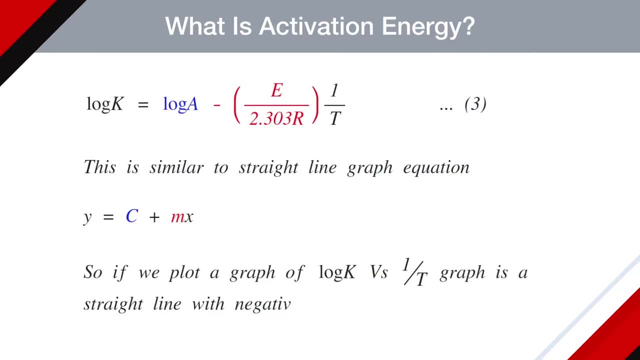 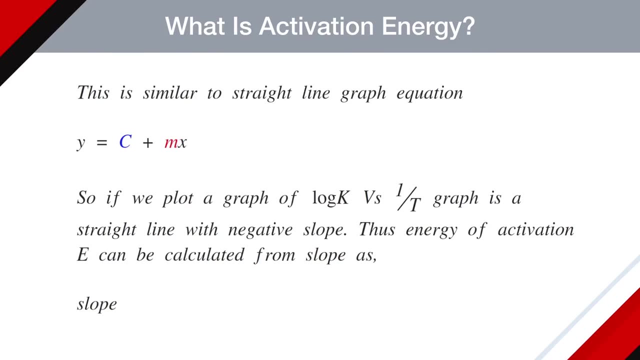 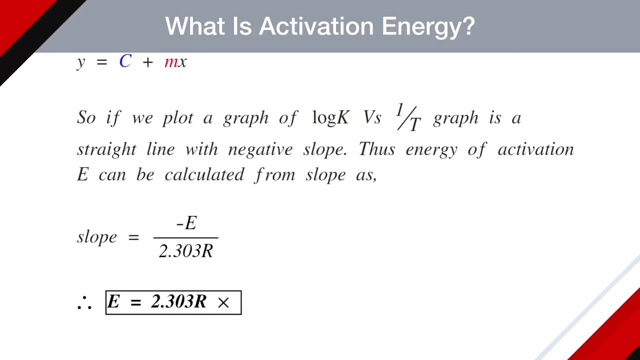 versus 1 by t. graph is a straight line with negative slope, Thus. Thus, energy of activation E can be calculated from slope, as slope is equals to minus E by 2.303 R. therefore, energy of activation E becomes 2.303 R into negative slope. 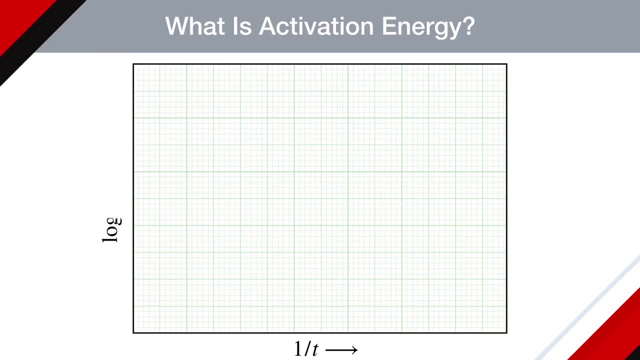 So you can see here as we plot a graph of log of K versus 1 by T, the slope is negative and slope is equals to minus E by 2.303 R. therefore E energy of activation becomes minus into slope, into 2.303 R. 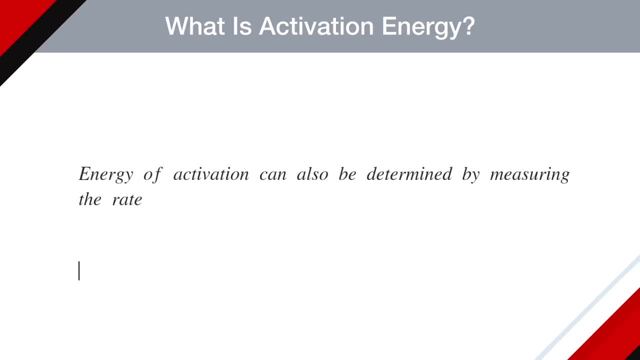 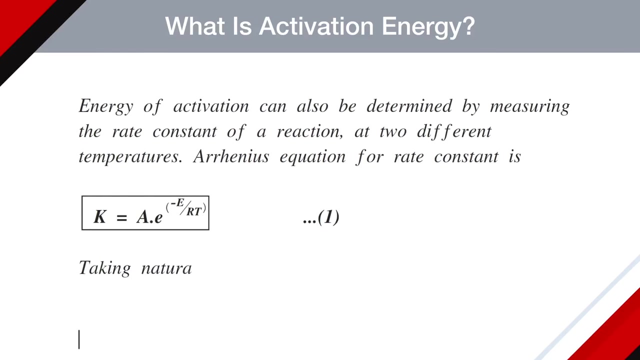 Energy of activation can also be determined by measuring the rate constant of a reaction at two different temperatures. Arrhenius equation for rate constant is: K is equals to A into E, to the power minus E by RT. this is equation number one. Taking natural log of both sides, we get ln. K is equals to ln of A into E, power to minus. 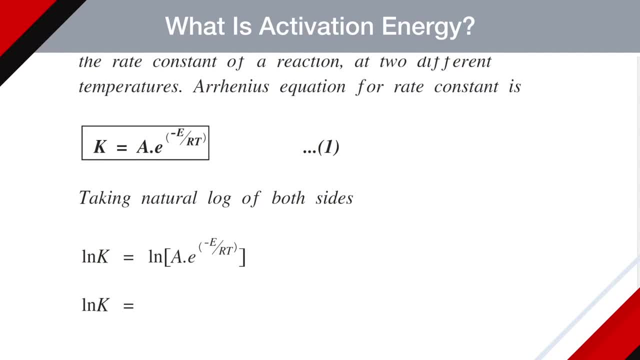 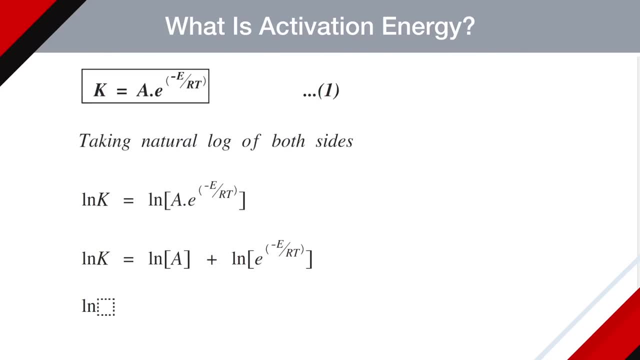 E by RT. Now let's expand the multiplication, so ln K becomes ln of A plus ln of E power to minus E by RT. Here ln and exponential gets cancelled, so ln K becomes ln A plus minus E by RT. or we can write: ln K is equals to ln A minus E by RT. this is equation number two. 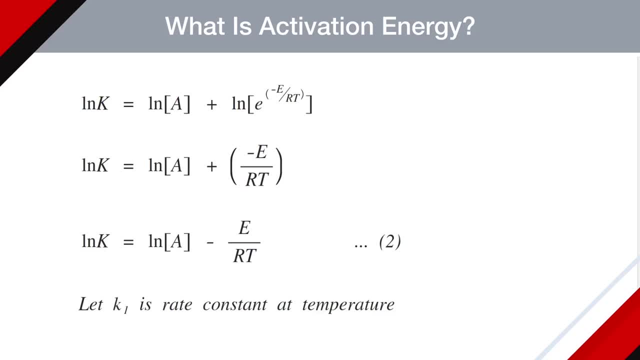 Let K1 is rate constant at temperature T1 and K2 at T2 respectively. So we can write: ln K is equals to ln A minus E by RT. this is equation number two. Let K1 is rate constant at temperature T1 and K2 at T2 respectively. 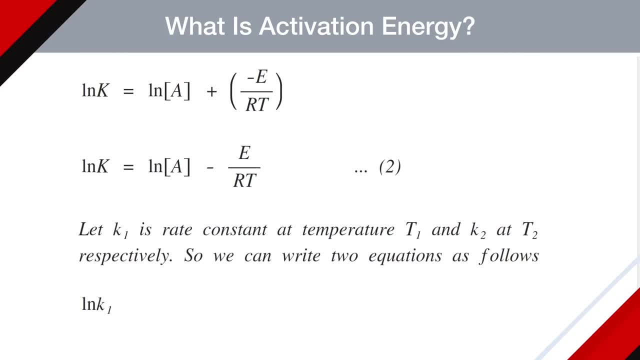 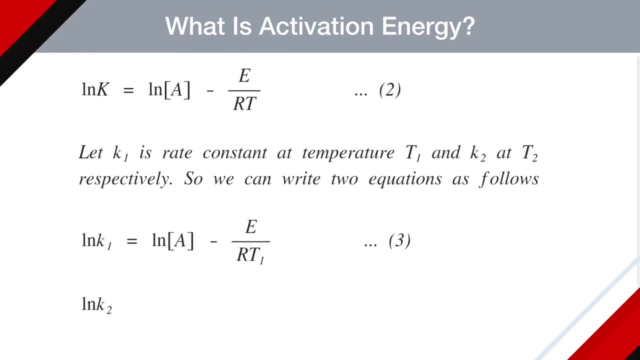 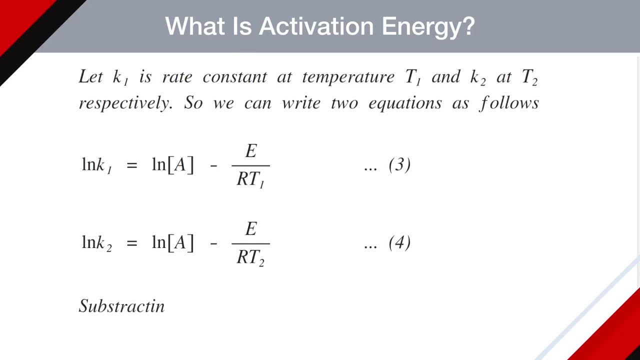 So we can write two equations as follow: like ln K1 is equals to ln A minus E by RT1- this is equation number three- and ln K2 becomes ln A minus E by RT2- this is equation number four. Now, subtracting equation three from equation four, we get ln K2 minus ln K1 is equals to: 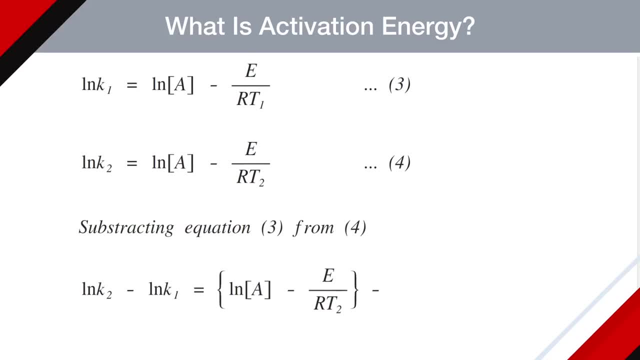 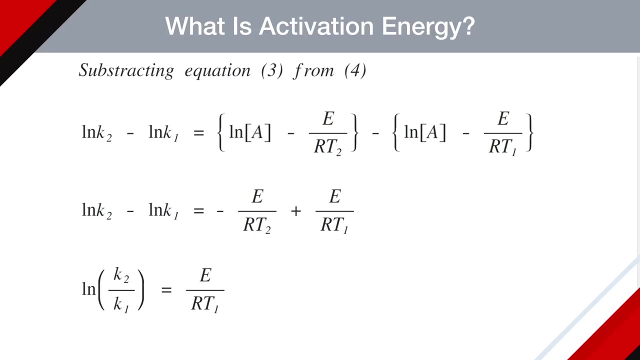 ln of A minus E by RT2, minus ln of A minus E by RT2.. Here ln of A factor gets cancelled, so equation becomes: ln of K2 minus ln of K1 is equals to minus E by RT2 plus E by RT1. or we can write down: ln K2 by K1 is equals to E by RT1 minus. 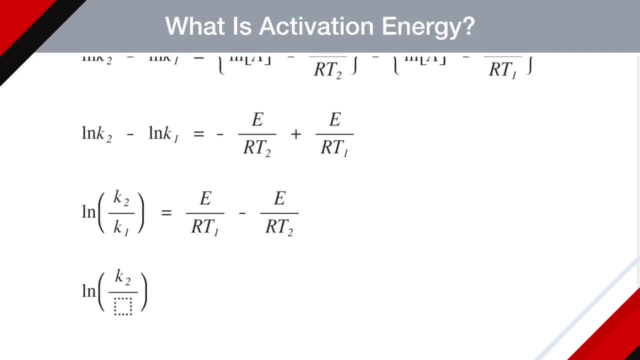 E by RT2.. In simple words, ln of K2 by K1 is equals to E by R, 1 by T1 minus 1 by T2. this is equation number five. Now again, natural log can be converted into log to base 10 as 2.303 log of K2 by K1 is. 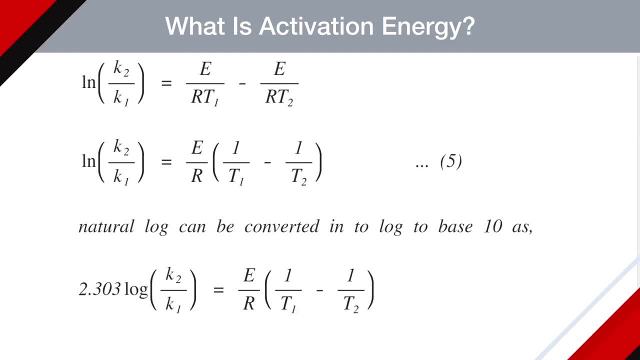 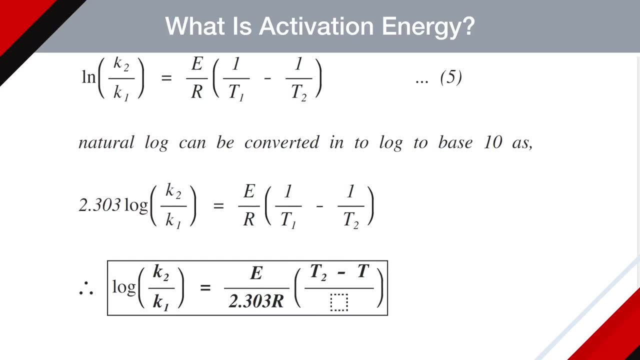 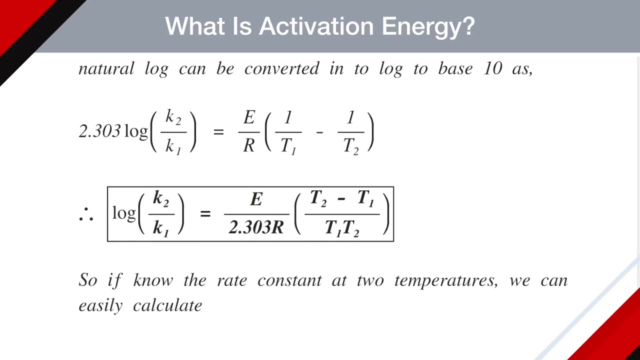 equals to E by R, 1 by T1 minus 1 by T2.. Therefore log of K2 by K1 becomes E by 2.303 R T2 minus T1, divided by T1 into T2.. So from this equation, if we know the rate constant at two temperatures, we can easily 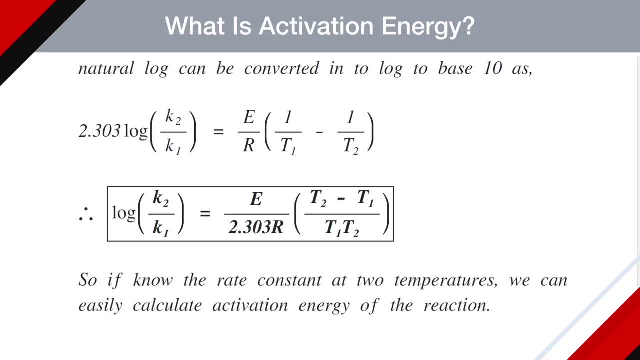 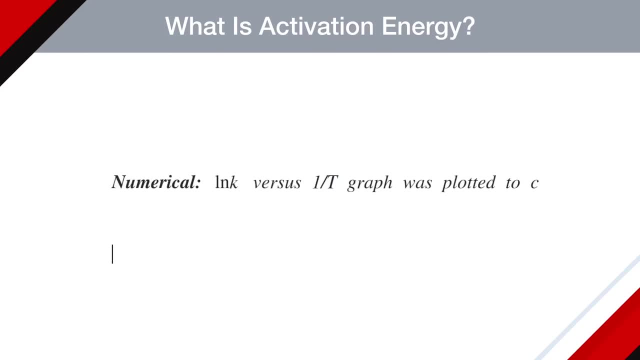 calculate activation energy of the reaction. So now let's look at the next equation. Let's look at the next equation. Let's look at the next equation. Let's try to solve a numerical based on this equation: ln, K versus 1 by T, graph was plotted. 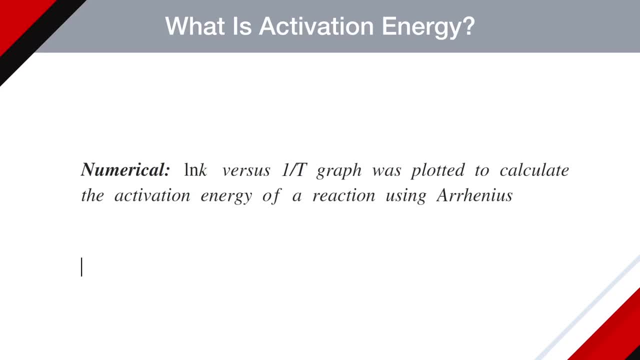 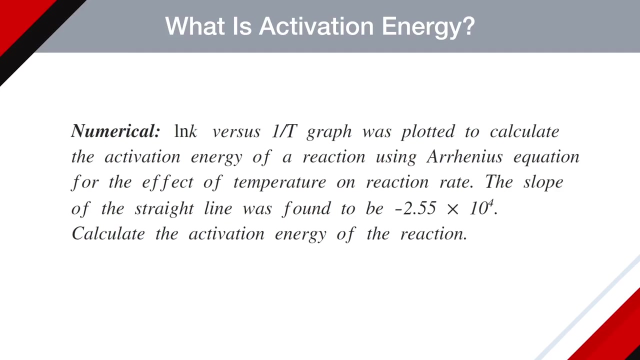 to calculate the activation energy of a reaction using Arrhenius equation for the effect of temperature on reaction rate. The slope of the straight line was found to be minus 2.55 into 10 to the power 4 calculate the activation energy of the reaction. in this case, slope of the graph is given, which is: 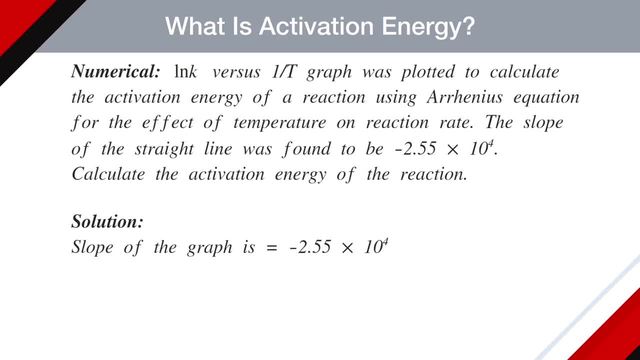 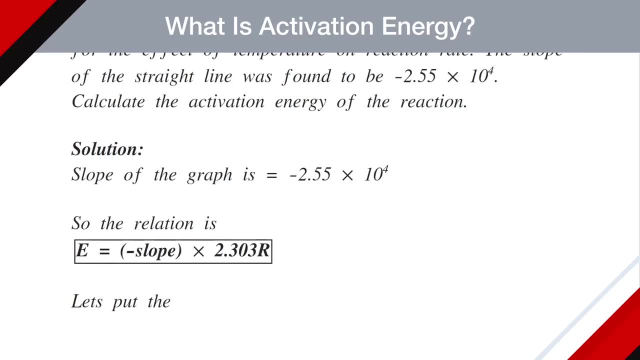 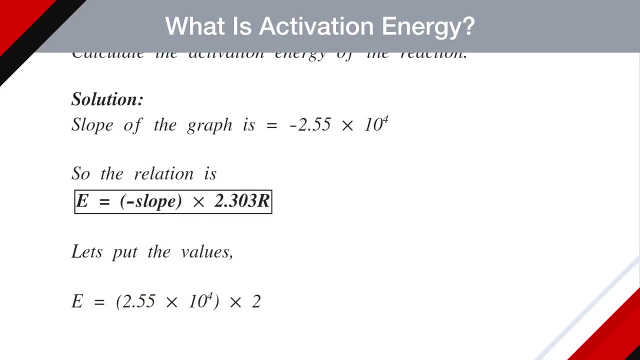 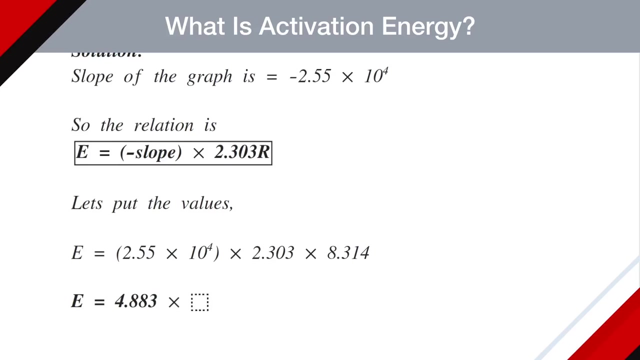 minus 2.55 into 10 to the power 4.. So from the equation E is equals to minus slope into 2.303 R. let's put the values minus. minus gets cancelled. So E becomes 2.55 into 10 to the power 4 into 2.303, into 8.314, which comes 4.883 into 10. 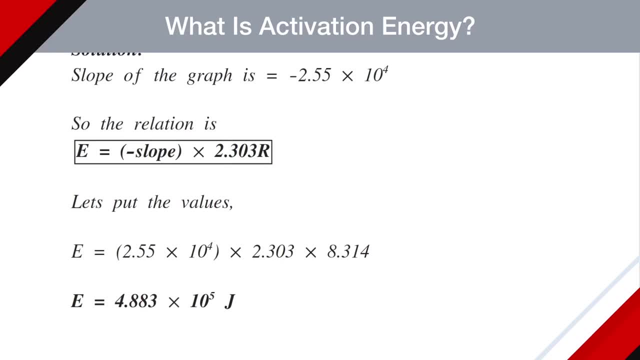 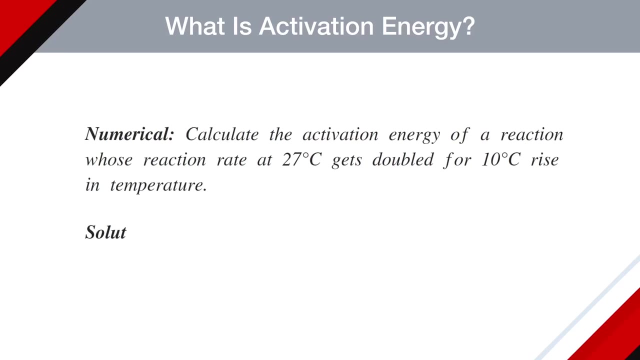 to the power 5 joules. So let's try another problem with the similar equation. So calculate the activation energy. The activation energy of a reaction whose reaction rate at 27 degrees Celsius gets doubled for 10 degrees Celsius rise in temperature. In this case two temperatures are given and the rates are also given and we have to calculate. 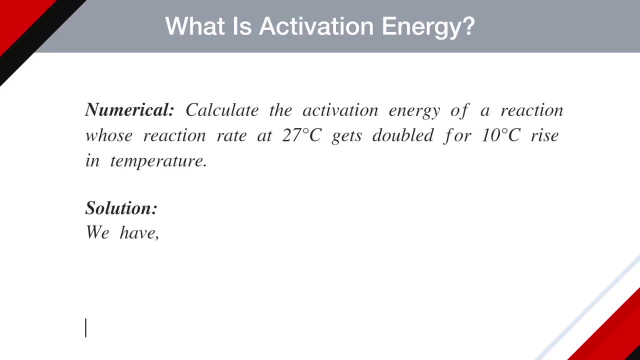 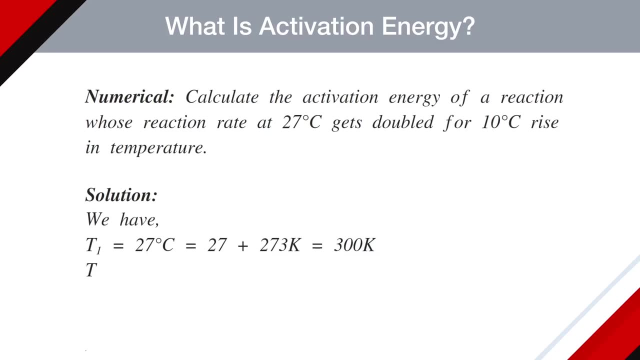 the activation energy. So T1 is 27 degrees Celsius, which is 27 plus 273 becomes 300 degrees Kelvin. and the second temperature is rise of 10 degrees Celsius. So T2 is equals to 27.. Plus 10 degrees Celsius, which becomes 37 plus 273, it becomes 310 degrees Kelvin. and also 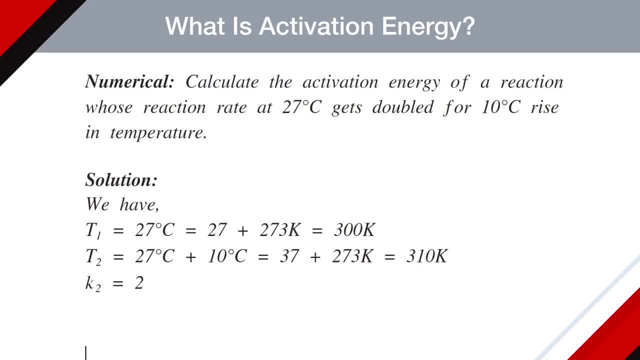 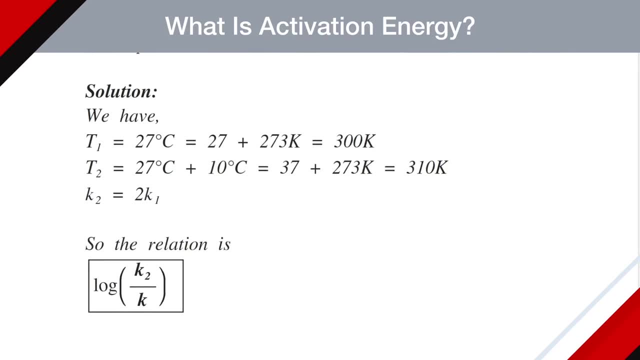 rate constant gets doubled. that's why K2 is equals to two times of K1 and the relation with two temperatures is given as log of K2 by K1 is equals to E by 2.303 R T2 minus T1 divided by T1 into T2.. 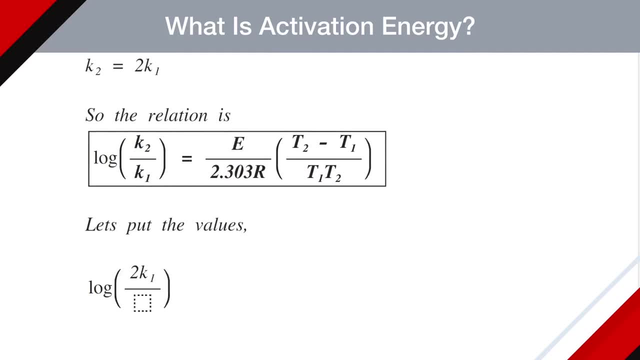 Let's substitute the values. So log of 2K1 divided by K1 is equal to T2 minus T1 divided by T1 into T2.. So log of 2K1 divided by K1 is equal to T2 minus T1, divided by T1 into T2.. 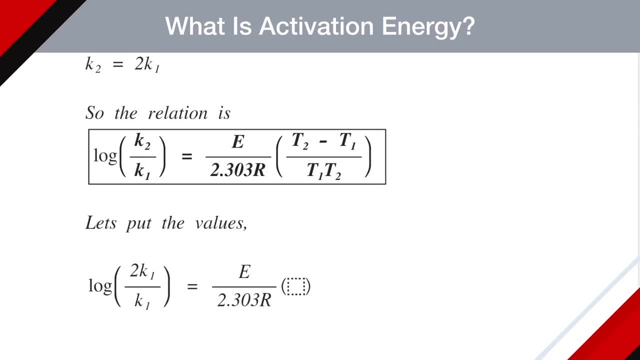 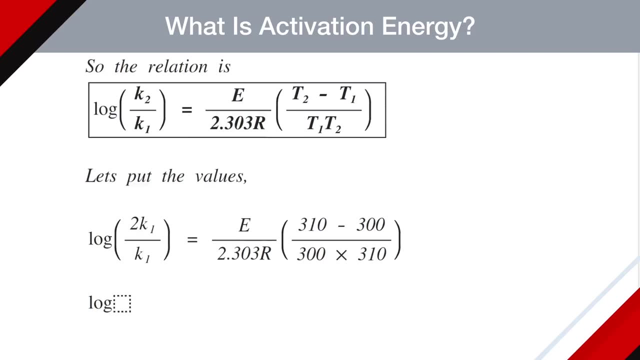 Let's substitute the values. So log of 2K1 divided by T2 equals to E divided by 2.303 R 310, minus 300 divided by 300 into 310.. So K1 gets cancelled and log of 2 is equals to E divided by 2.303 R 10 divided by 93000. 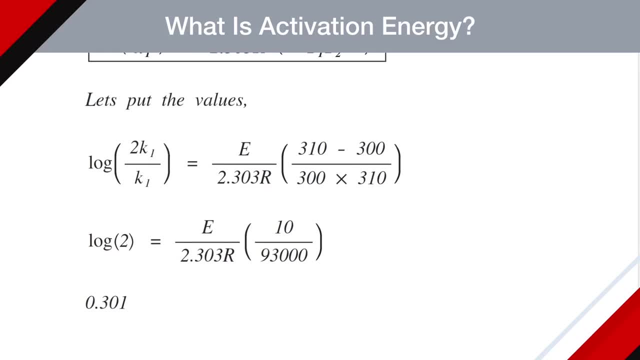 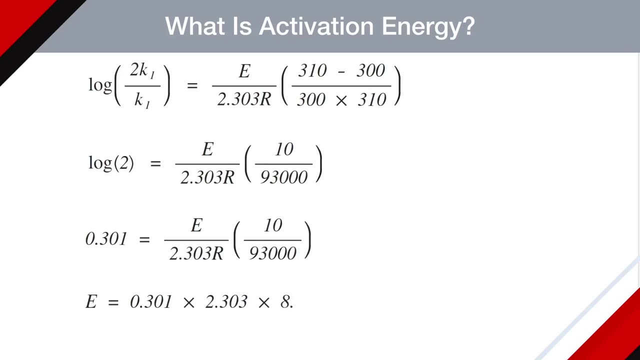 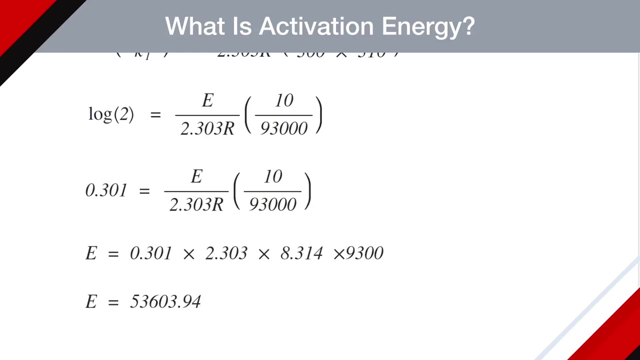 or 0.301, is equals to E divided by 2.303, R into 10 divided by 93000.. On rearranging equation, E becomes 0.301.. Let's substitute this 0.301 into 2.303, into the value of R8.314, into 9300.. So E becomes 53603.94 joules per. 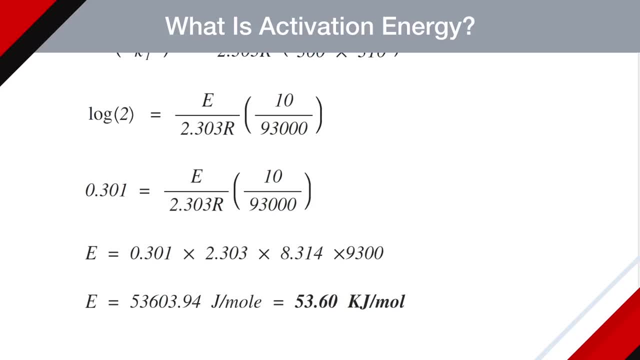 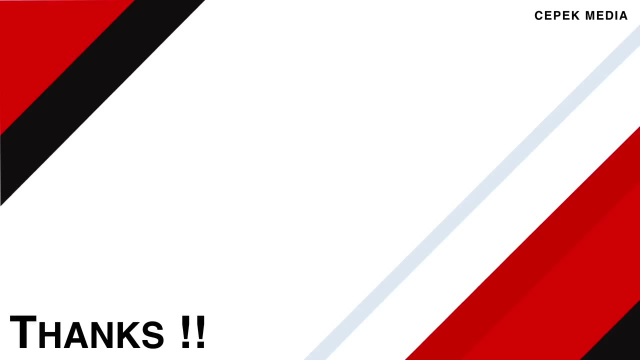 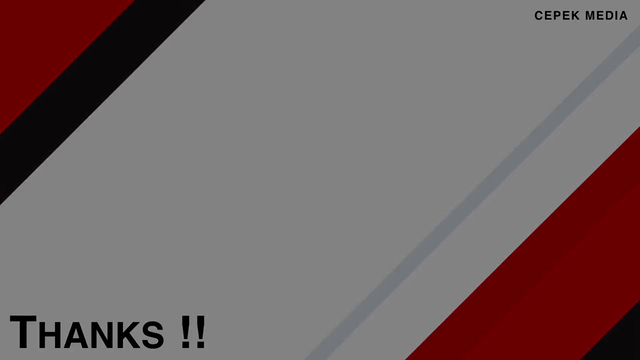 mole, or we can say 53.6 kilojoules per mole. If you like this video, please click on the like button and also subscribe to this channel. Thank you so much. Thank you.